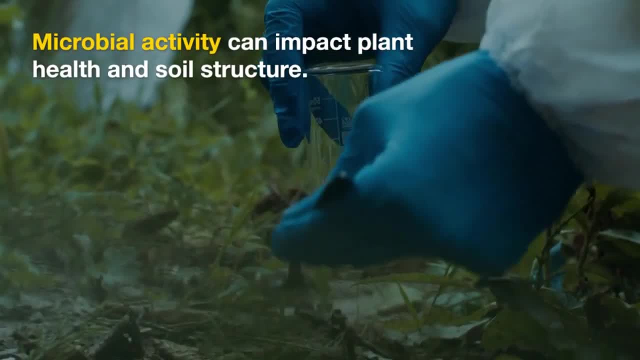 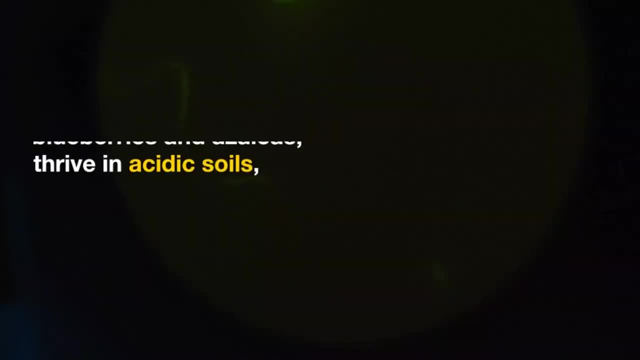 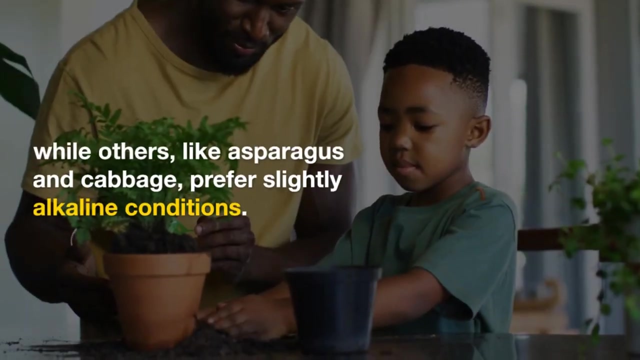 Microbial activity can impact plant health and soil structure. 4. Plant Growth and Development. Different plants have varying preferences. Some plants, like blueberries and azaleas, thrive in acidic soils, while others, like asparagus and cabbage, prefer slightly alkaline conditions. 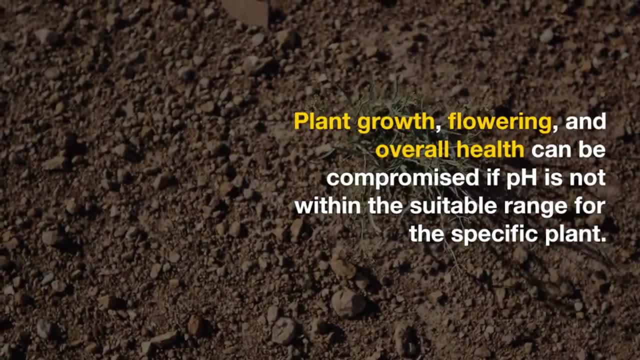 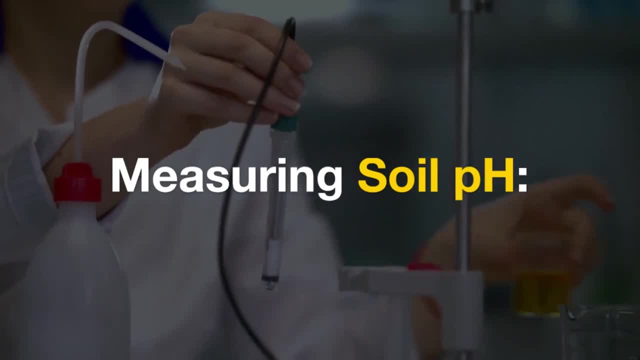 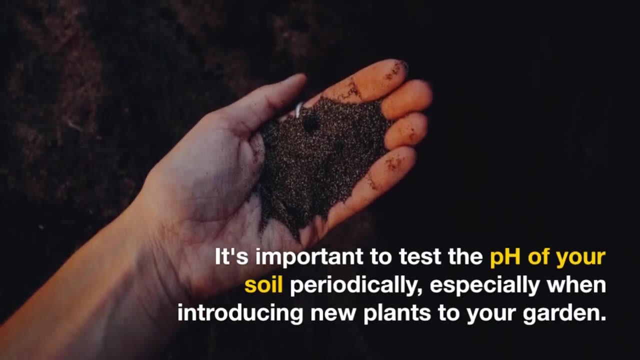 5. Plant Growth. Plant growth, flowering and overall health can be compromised if pH is not within the suitable range for the specific plant. Measuring Soil Each You can measure soil pews in a soil pesting kit. It's important to test the pH of your soil periodically. 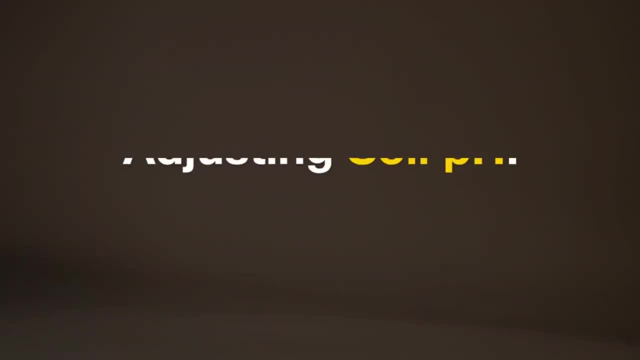 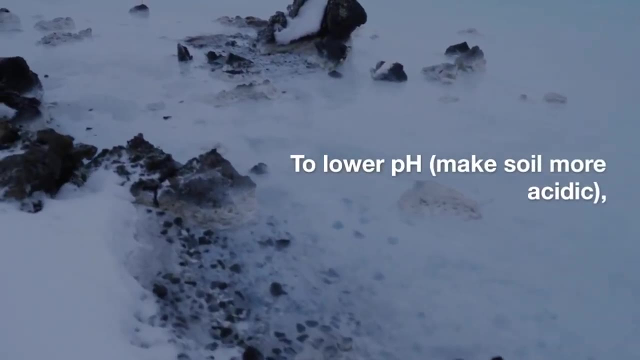 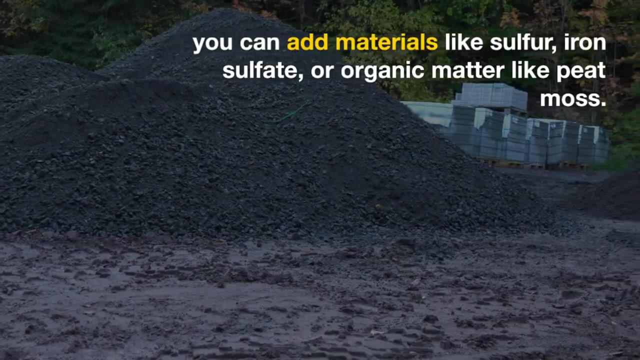 especially when introducing new plants to your garden. Adjusting Soil: 1. Acidifying Soil To lower pay. make soil more acidic. You can add materials like sulfur, iron sulfate or organic matter like peat moss. Be cautious when using sulfur. Excessive use can lead to soil imbalances. 2. Alkalizing Soil. To raise P, make soil more alkaline. You can add materials like lime, calcium carbonate or wood ash. Adjust the amount of lime based on the current pay and the target page. 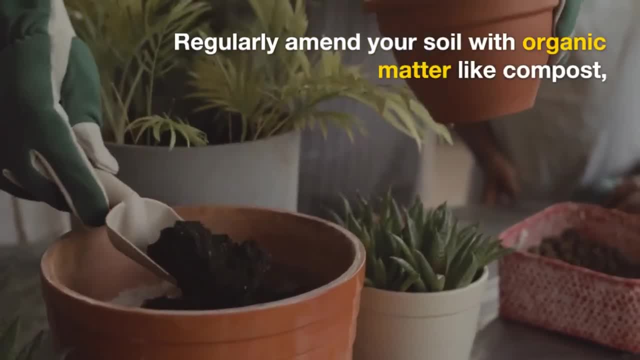 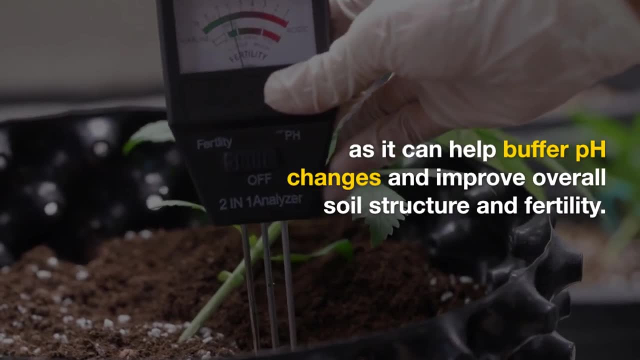 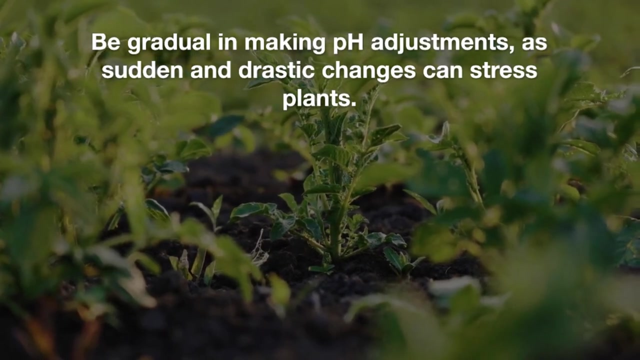 3. Alkalizing Soil: General Tips. Regularly amend your soil with organic matter like compost, as it can help buffer peach changes and improve overall soil structure and fertility. Be gradual in making pH adjustments, as sudden and drastic changes can stress plants. 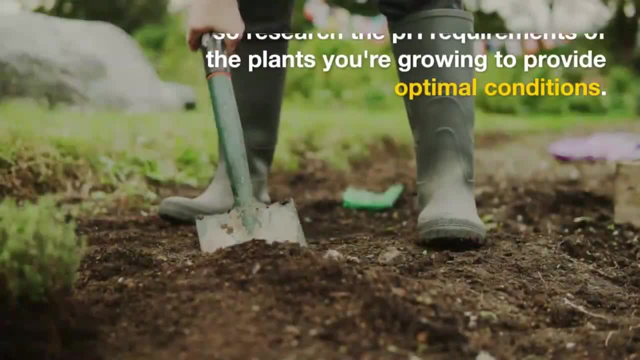 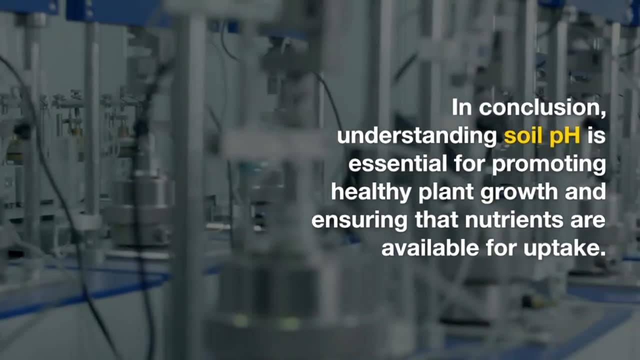 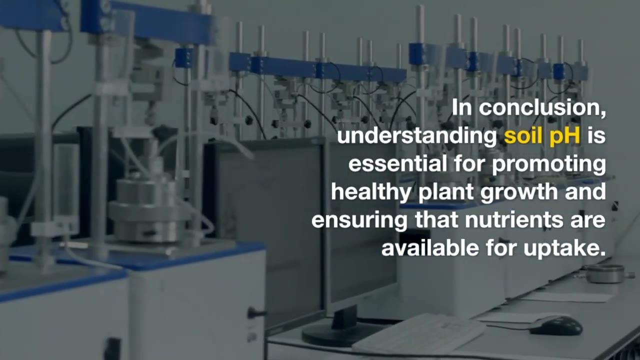 Different plants have different preferences, So research the pH requirements of the plants you're growing to provide optimal conditions. 4. Planting and growing plants. In conclusion, understanding soil pH is essential for promoting healthy plant growth and ensuring that nutrients are available for uptake. 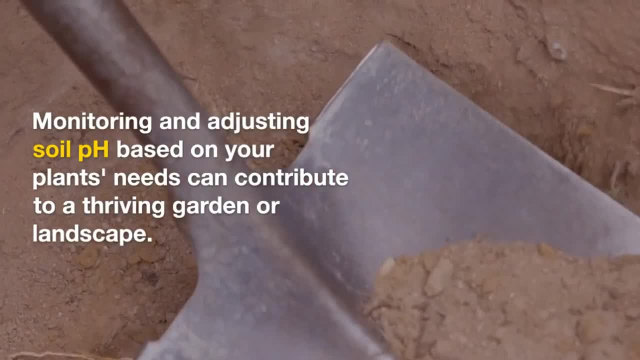 Monitoring and adjusting soil pH based on your plant's needs can contribute to a thriving garden or landscape.